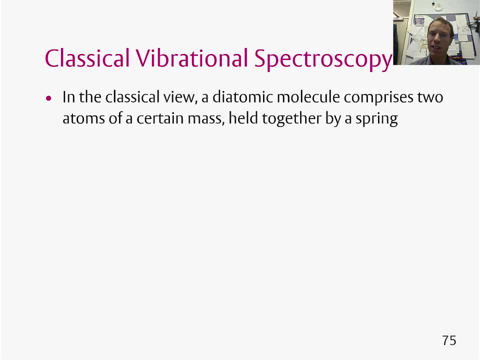 classically you have the view of a diatomic molecule as being two atoms of certain mass held together by a spring. This spring has a certain stiffness, a certain force, constant and an equilibrium length. So we can draw a molecule something like this: So we have a mass. 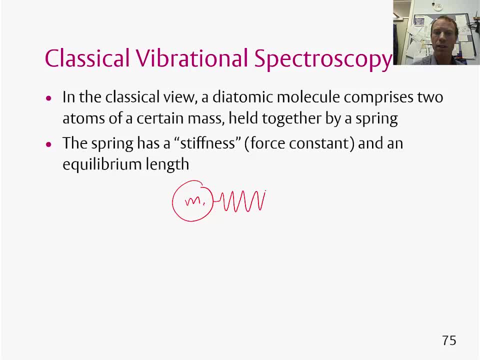 1, one atom, we've got a spring, and then another atom of mass m2.. This spring has a force constant, k, and an equilibrium length, re. If you now stretch or compress this molecule, the spring creates a restoring force which is proportional to the magnitude of the displacement. So we can write this expression here. So where? 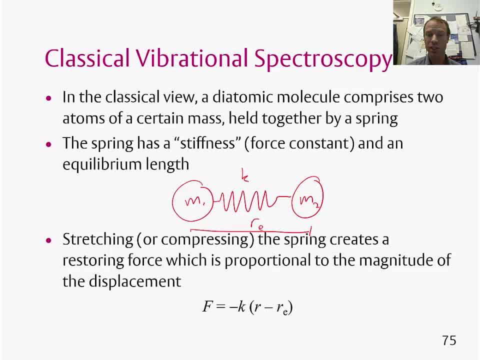 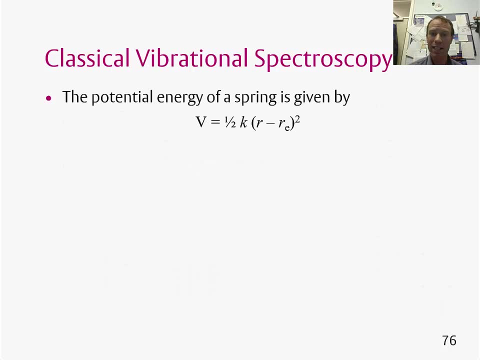 the force is equal to minus k, where k is the force constant multiplied by r minus re, where re is the equilibrium bond length of the molecule. The potential energy of a spring is then given by this expression here. So we've seen: k is the force constant, re is the equilibrium bond length. 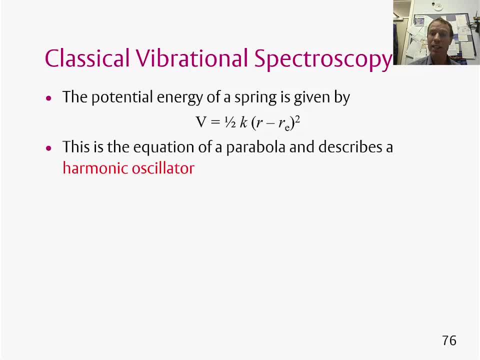 This is actually the equation of a parabola and describes a so-called harmonic oscillator. So a harmonic oscillator potential looks like this: So we have potential energy up the left, we have bond length on the x-axis and we have this curve. This is how a spring behaves and if you have a spring, 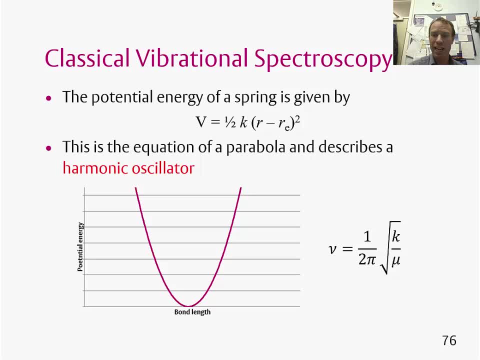 with a reduced mass of mu and a force constant k. so here we have mu, here we have k. then the vibrational frequency of this spring is given by nu, the Greek letter nu. So if you know the force constant, you know the reduced mass, you can work out what the natural vibrational 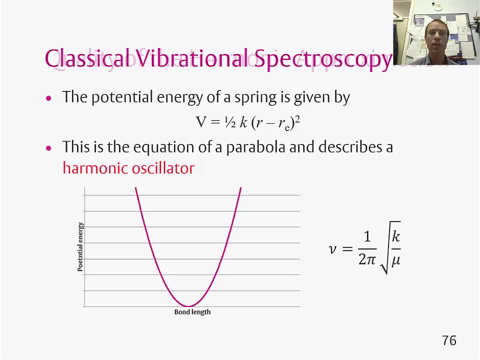 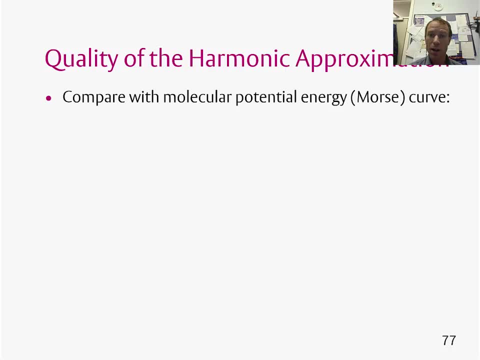 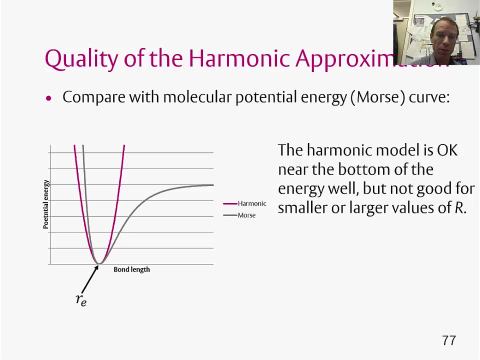 frequency is The harmonic approximation is only an approximation though, So real molecules are better described by a Morse curve. So here we have a plot where the harmonic potential is in pink and the Morse curve is in grey, And you can see that the harmonic model is okay around the bottom. 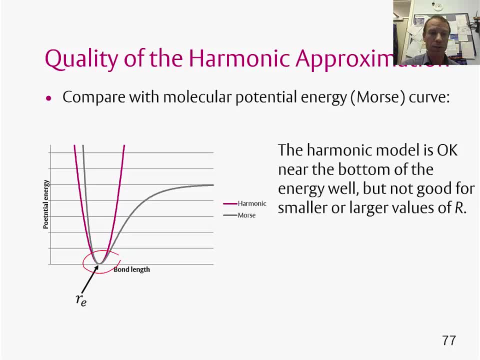 of the well. so if we're down here, the harmonic model is quite good, But if we go up to higher energy? so here we can see that the harmonic model is actually not very good. We'll see a correction factor for this later on. 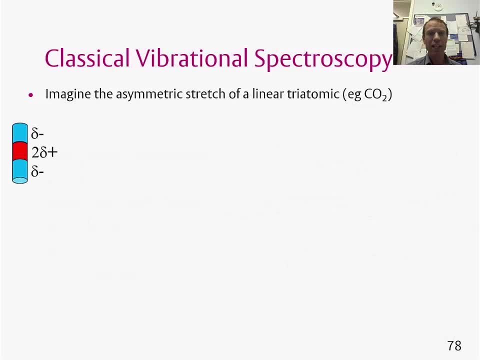 So we've thought a bit about the vibrations of a spring. How does a vibrating molecule interact with light? So here's a classical picture of what's going on in vibrational spectroscopy. If we can imagine a linear triatomic such as CO2,, this has a delta plus and a delta. 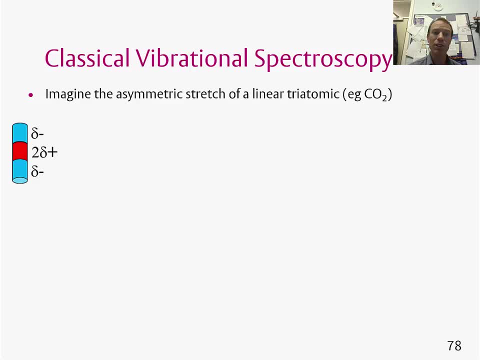 minus. And if you think about the asymmetric stretch, so as one bond gets longer the other bond gets shorter, So it looks something like this: We can now think about the dipole moment of this molecule. So initially there's no dipole. 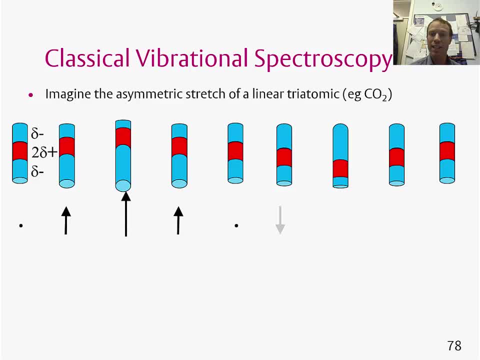 moment, but then it gets bigger and points in one direction, and then it gets bigger and points in the other direction. If we were to plot this on a graph, as a function of time we get a nice curve, And in the same way as when you were looking at rotations, if we've 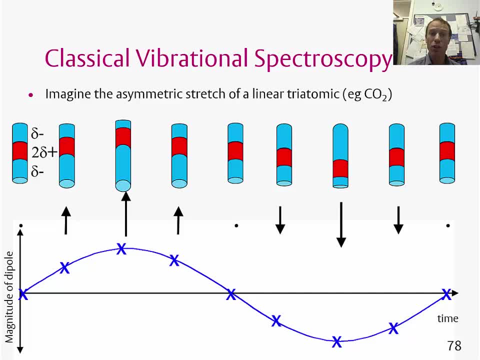 got an oscillating curve. we get a nice curve. And if we were to plot this on a quantitative graph, we get a nice curve. And in the same way as when we were looking at rotations dipole, this will then interact with the oscillating electric field of light. so 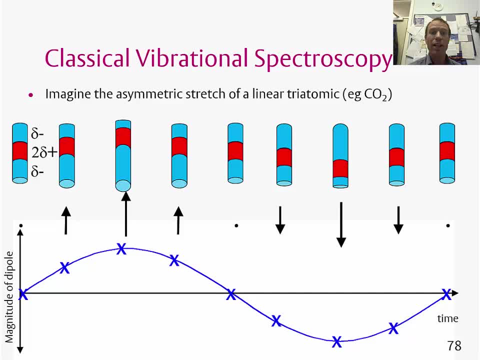 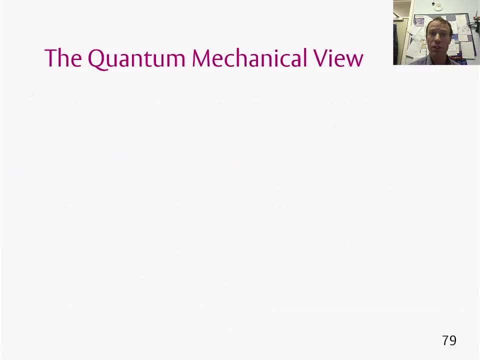 this is how vibrational spectroscopy works. you'll have to remember this is just a classical picture, so it doesn't give us all the details we need, but it helps us get a feel for what's actually going on. of course, to understand what's going on, we need we need to go to quantum mechanics so we can solve the 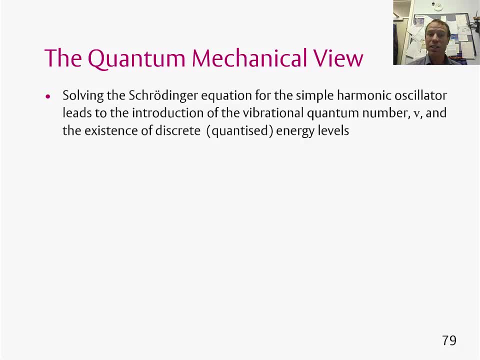 Schrodinger equation for a simple harmonic oscillator, and this leads to the introduction of vibrational quantum number, of a vibrational quantum number V, and the existence of discrete energy levels. so if we have our harmonic potential, it looks something like this: we'll now get energy levels. 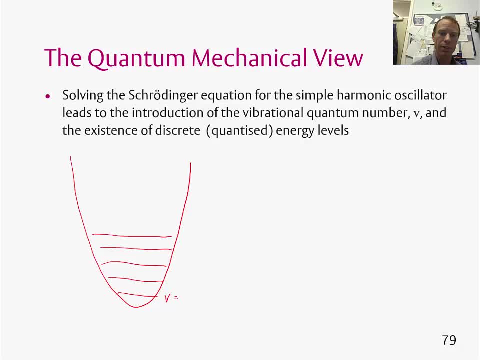 with different V. so this is V equals zero. this is V equals zero equals one, equals two, equals three, equals four, and so on. the energy in joules of one of these vibrational wave on one of these vibrational states is given by this expression here. here we've got H. so Planck's constant new the. 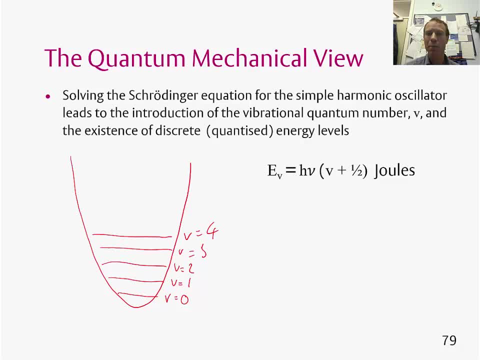 vibrational frequency, and we've got V, the quantum number. you can see, we've got to be very careful to distinguish between news and V's. so first of all you need to get them clear in your mind, what they and they mean, and then make sure that when you write them, 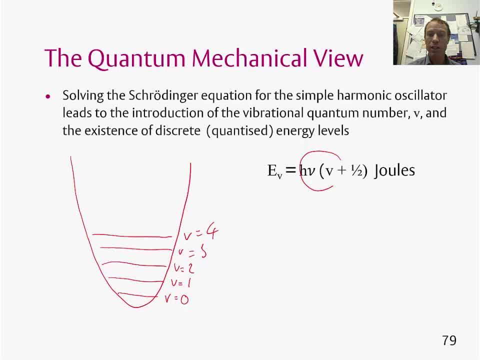 you're also very clear. we can express this in terms of a vibration wave number, new tilde, and that gives us this expression here for the energy of these states. one of the very interesting things that happens when you solve the Schrodinger equation for a simple harmonic oscillator is you get so-called 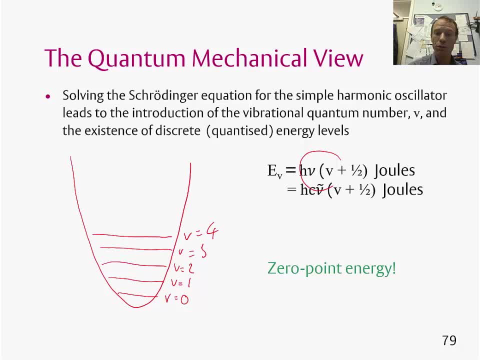 zero point energy and zero point energy, often abbreviated to ZPE, is this energy gap here. the interesting thing here is that the lowest possible vibrational state doesn't have zero energy. it's got a finite, nonzero energy and this is described by zero point energy. this is a purely quantum mechanical effect and 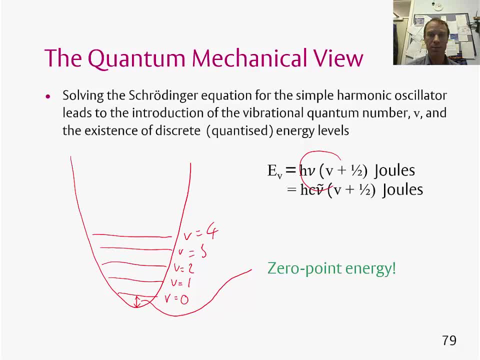 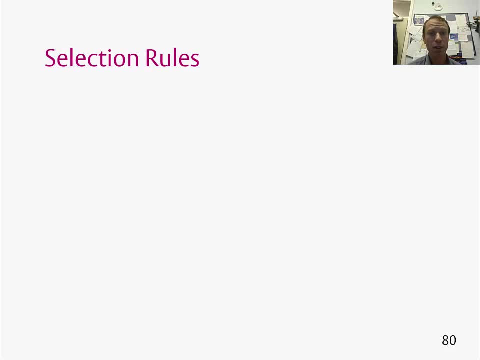 it doesn't doesn't happen in a classical case. okay, so we've understood a little bit about what's going on, how light interacts with a vibrating molecule and how solving the Schrodinger equation gives rise to vibrational energy levels. we now need to think about the selection rules which account for. 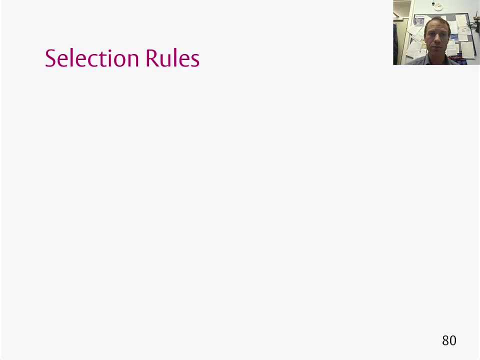 transitions between these energy levels. as always, we've got a global rule and a specific rule here. the global rule is that the energy levels of the energy is that there must be a change in the electric dipole of the moment dipole of the molecule during the vibration. so an example could be a linear molecule like 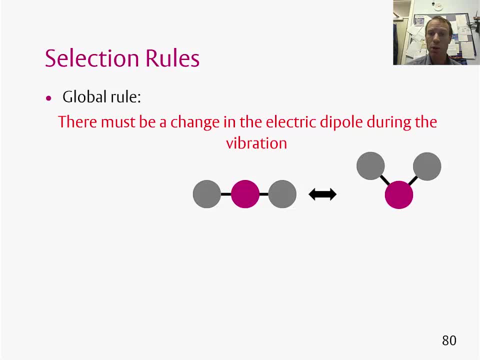 co2, if it bends one way and the dipole moment will point one direction, and if it bends the other way, then the dipole moment will point in the other direction. so this is a case where this this happens. the specific rule for vibration absorption spectroscopy is delta. v equals plus or minus one. so this says that v. 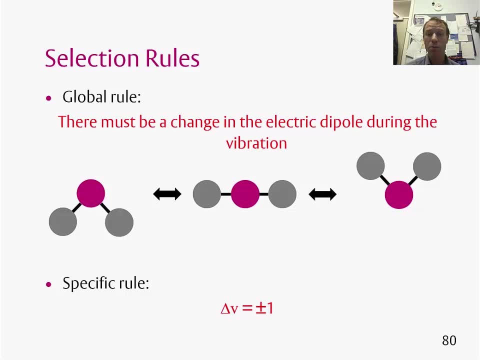 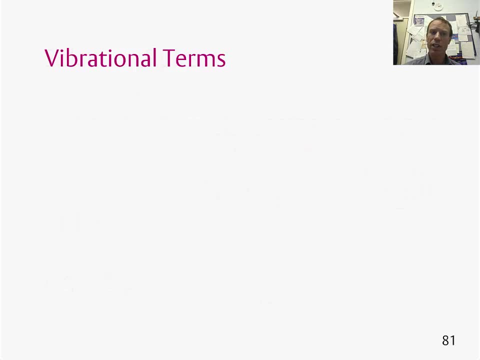 the vibrational quantum number can change by plus or minus one in a transition. we can also work in terms of vibrational terms, and this is working in with units of centimeters, to the minus one, working in in wave numbers rather than joules, so the wave number of a specific level. 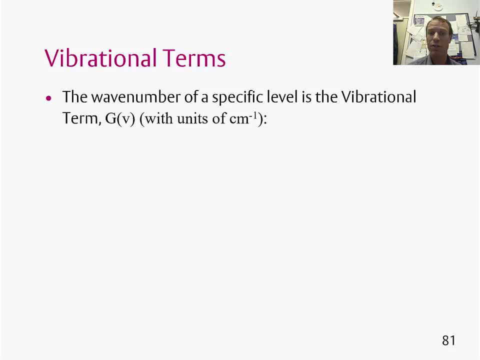 can be written as the vibrational term g of v, and this has units of centimeters to the minus one. so we get a vibration wave number from an energy in joules by dividing by h c. so if you remember the expressions from a couple of slides back, we can now write: g of v equals nu tilde multiplied. by hc. so what this method has done is it has modified the expressions. so we've changed all g of v details and the expressions now worked by plutonily Sum over hc, so because of minute toplum. So how can we change out to an energy dot dotTime relationships? 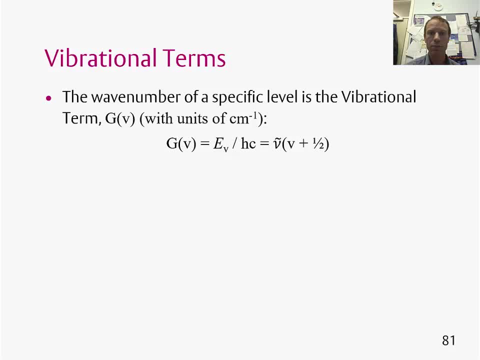 V plus a half in this expression. here we know from the selection rules that an allowed transition is Delta J. Delta V- sorry- is plus or minus one, so we can get the wave number of a transition. so a transition wave number of a loud transition is therefore just equal to nu tilde. so it's very simple expression. 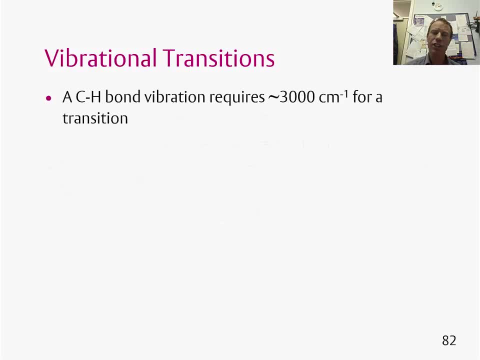 let's think about vibrational transitions and how many peaks we'd expect to get in a spectrum. if you think about a CH bond, they come at around 3,000 centimeters to the minus one in a infrared spectrum and 3,000 centimeters. 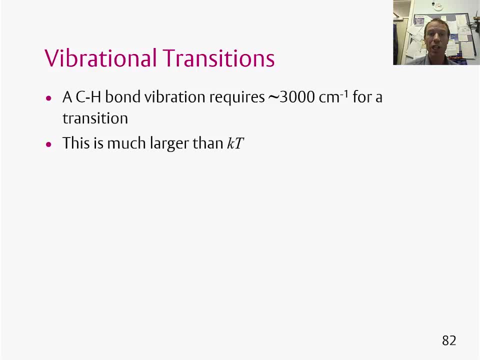 to the minus one is much larger than KT at room temperature. remember right back to the beginning of this course, when you were thinking about KT at different temperatures as being a rule of thumb for how much energy is available. this means that at room temperature most transitions will start from the ground vibrational state, so the